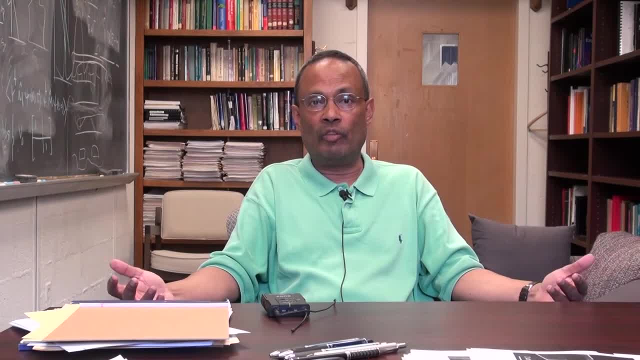 You can write down wave functions, and these wave functions seem to be very, very good. The way you know they're very, very good is that you can do numerical work, Or you can look at experiments and you find out the fractions that show up precisely. 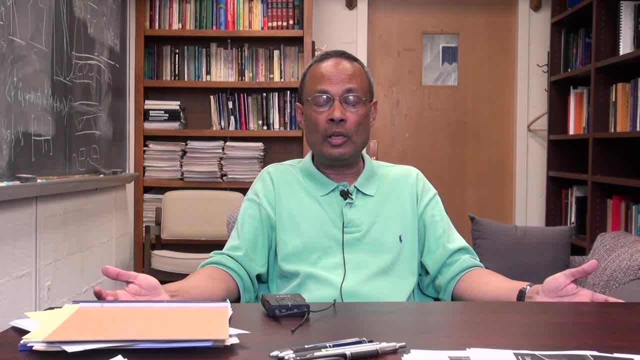 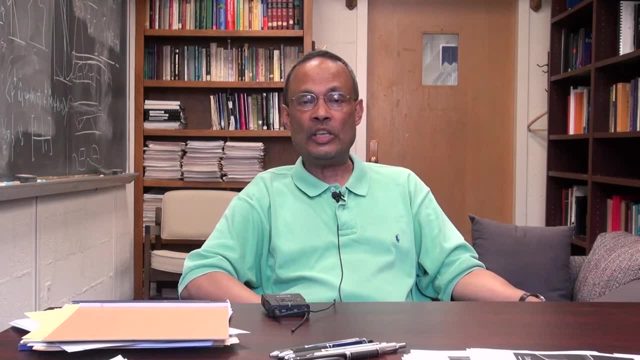 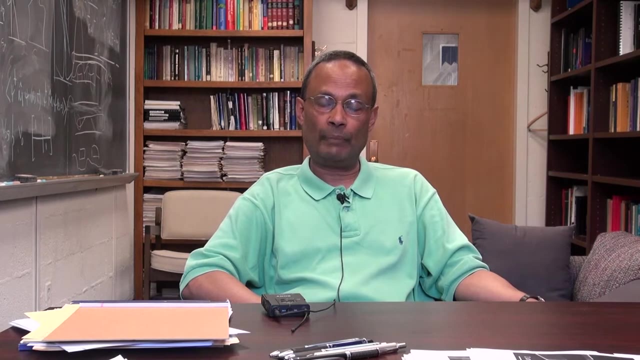 are the ones you get from this composite fermion prescription, and this is still very much an ongoing subject. But the main thing I want to talk about in this concluding speech, or lecture, whatever it is- is the exception to this odd denominator rule for fractional quantum Hall effect. 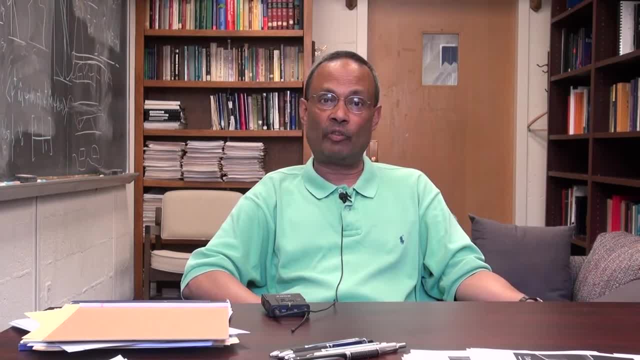 You know that fractional quantum Hall effect originally was seen at fraction one third, and then it was seen in many, many fractions of the nature of p over q, where q is always an odd number, And this odd number seems to be an unavoidable consequence of Pauli principle. 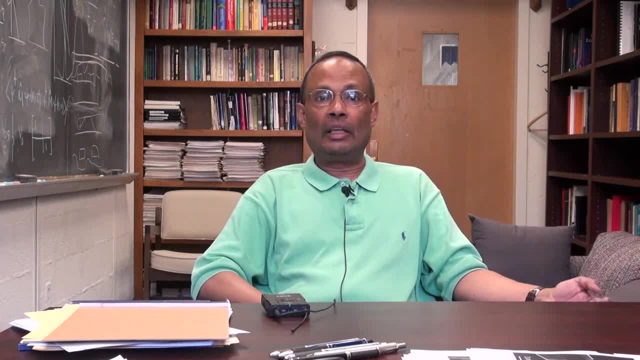 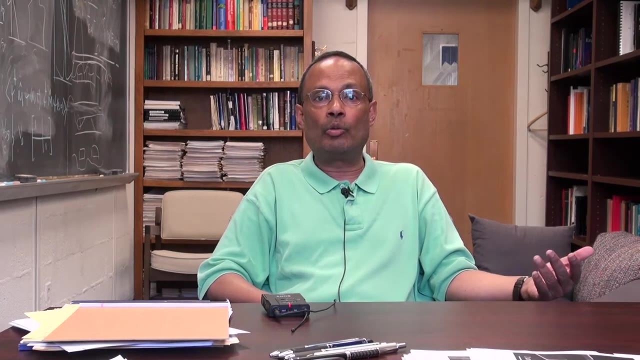 that electrons obey Pauli principle, so the wave function must have this form: that zi minus zj to the power m, where m is odd, z being the spatial coordinate of the electrons. So it seems that you cannot avoid it, because when zi is equal to zj, you must get a zero. 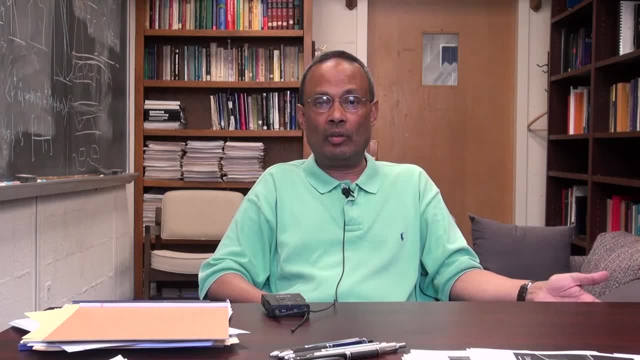 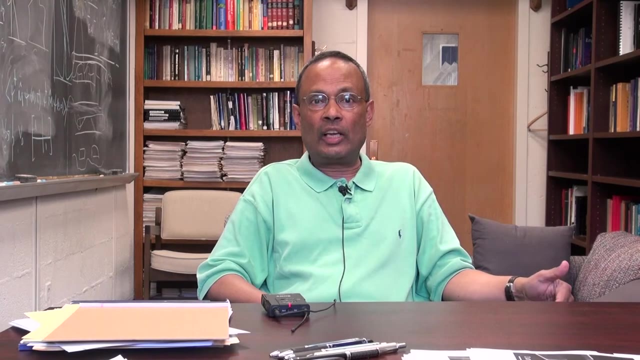 But amazingly, in 1987, almost thirty years ago, an even denominator fraction, specifically a fraction five over two, 2.5, two and a half, was seen. So what does it mean? I should add that no such fraction is seen at nu- is equal to half. 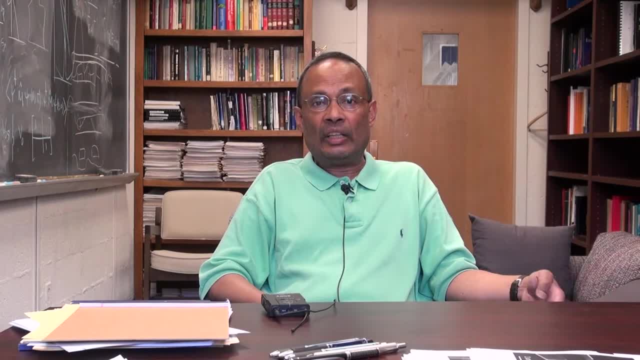 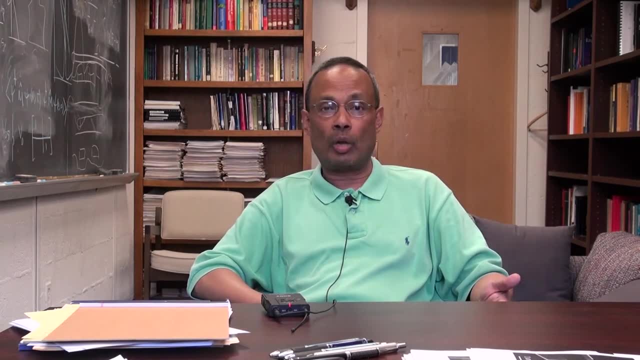 only at nu, is equal to five half and seven half. This turns out to be an effect which is as interesting as fractional quantum Hall effect itself. It's called even denominator fractional quantum Hall effect, And these objects are thought to be a strongly correlated system. 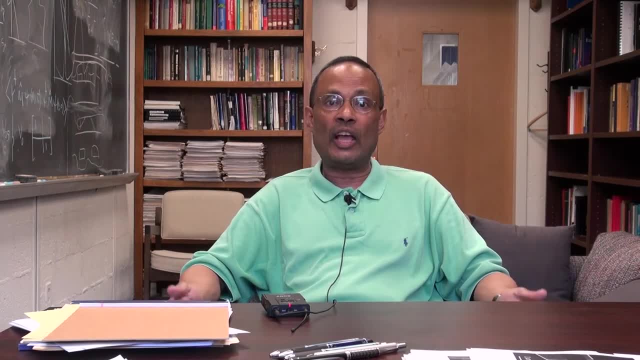 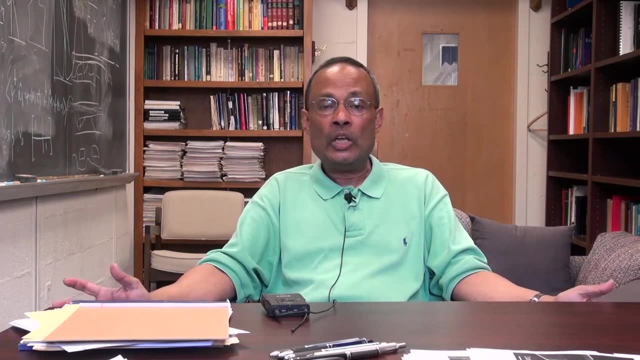 which is a spinless PUF superconductivity. You can write down wave function very similar to Laughlin wave function and Greg Moore and Nick Reed wrote this wave function down And this wave function has the form that the part, the polynomial part. 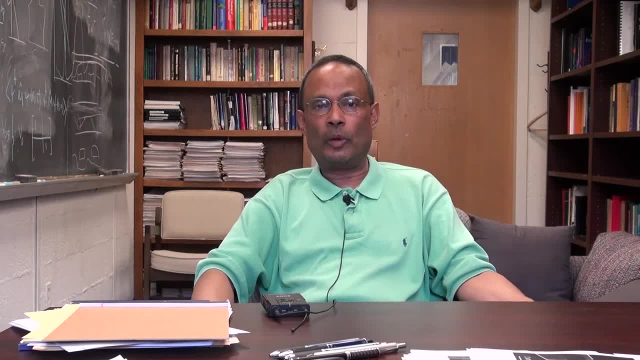 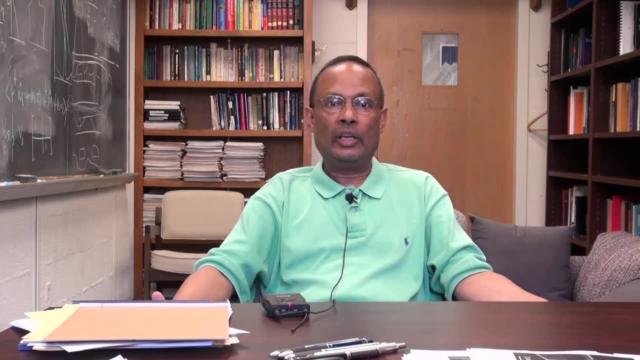 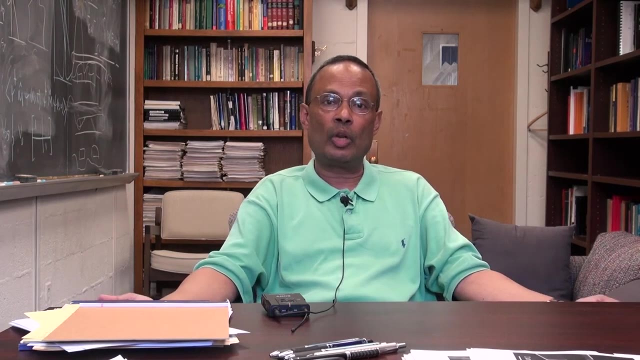 has zi minus zj to the power two, corresponding to five half that two. And of course they cannot be then electrons because they are essentially the wave function for P wave spinless superconductivity. In fact, the wave function that Moore and Reed wrote down is exactly the same.